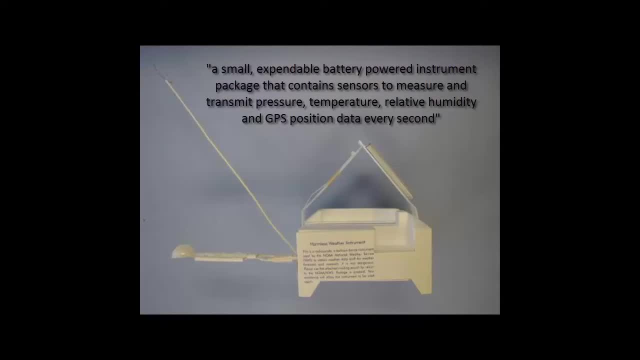 or NOAA. a radiosonde is a small, expendable, battery-powered instrument package that contains sensors to measure and transmit pressure, temperature, relative humidity and GPS position data every second. The boom seen going out at about a 45-degree angle, coming out of the 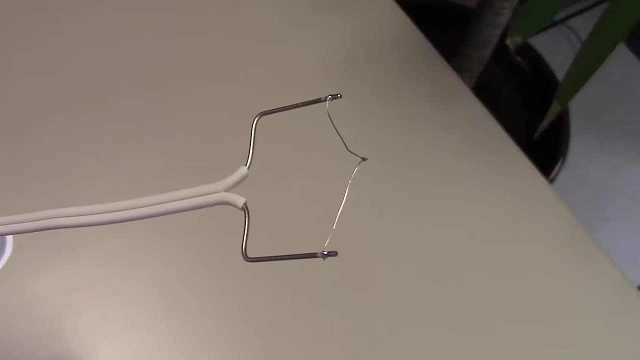 radiosonde body is called a thermistor. A thin rod comes out of the boom at the end, as seen here. Electrical resistance will change along the rod as the temperature changes, which is how we measure temperature values. The sensor on the left side of the radiosonde. 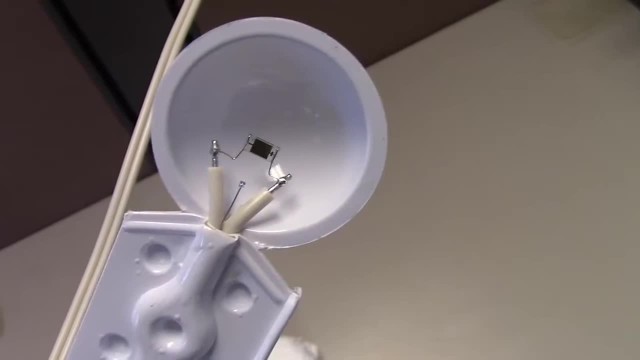 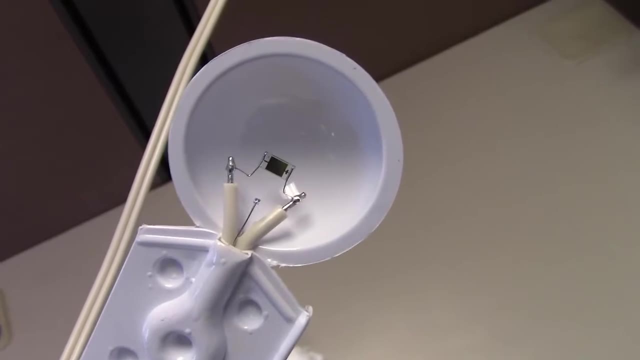 is called a hygristor, which measures relative humidity. This is done with a plastic piece that is coated with a celluloid resin and dried. This celluloid is sensitive to changes in humidity and the value is measured based on how much the sensor expands or contracts. 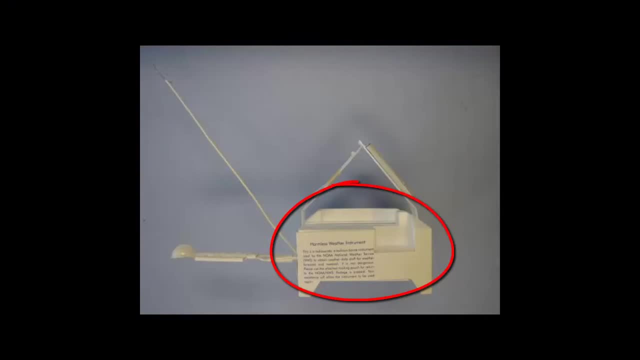 with the changing water vapor. The pressure and GPS sensors are located inside the radiosonde. Pressure is measured using a cell that will expand or contract in response to the changing pressureinner pressure measure is paramетров, which measures thekn Italy temperature by 2 to 5 gradations per second. uming temperature difference of 75,200 grandmother of bed last ideally 30 degrees to education20hours per minute and sensitivity 40 degrees per second. so a lot of. 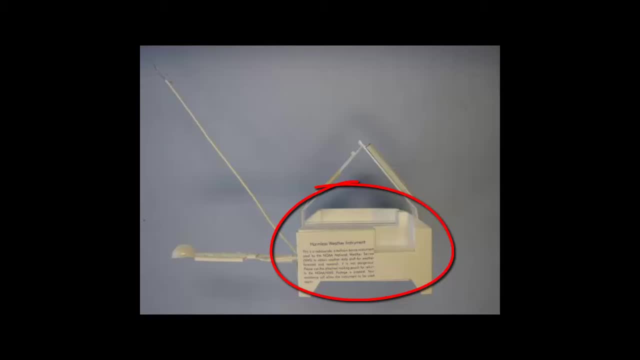 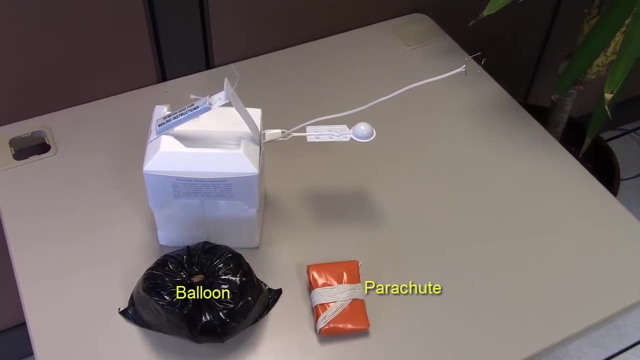 The GPS sensor inside will give location which the computer will then use for calculations of wind speed and direction. With the radio sign, we have our balloon and parachute which is used to help slow down the radio sign as it falls back to Earth. 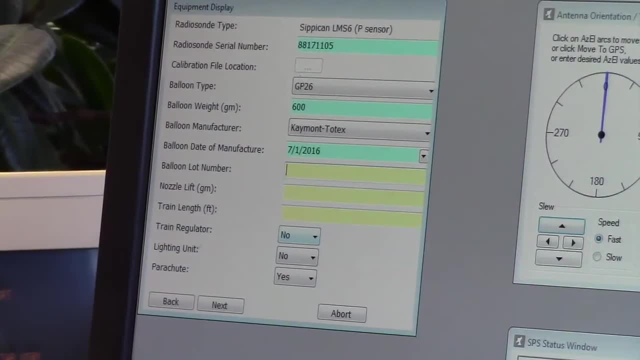 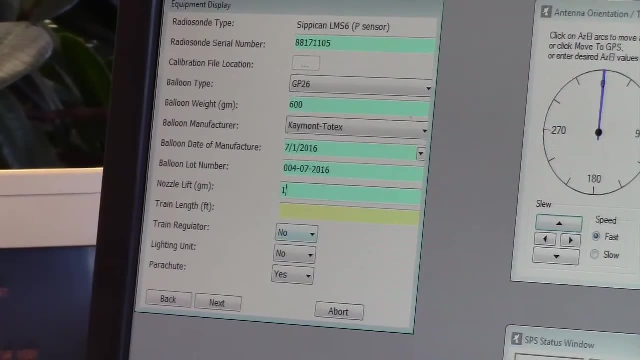 Before we begin launching we enter all of the necessary information into the upper air computer, which includes the radio sign, number, balloon type and how much gas will go into the balloon upon inflation. Then we enter in the current weather observations from the observing station outside the office. 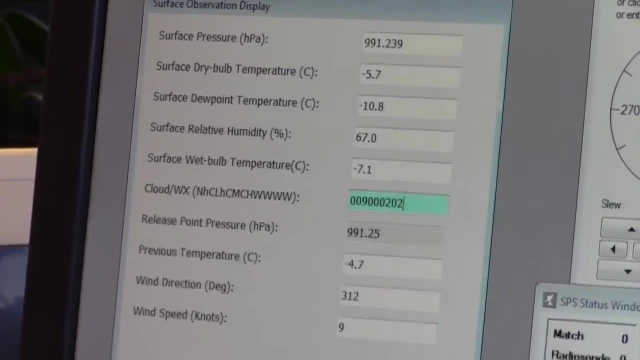 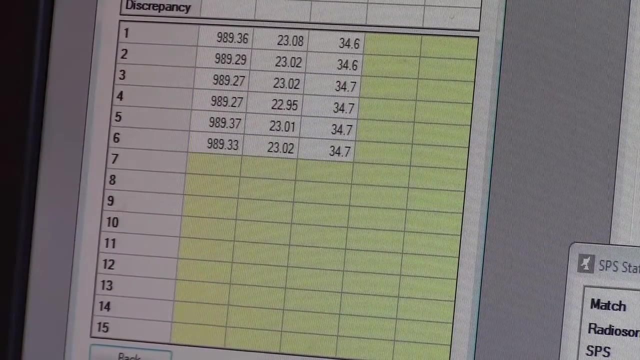 along with the cloud cover information and how that has been changing with time. We then can begin the process of baselining the radio sign, which is where we just ensure that the temperature, pressure and humidity sensors are working properly. We also want to make sure we are receiving an acceptable amount of GPS satellite matches. 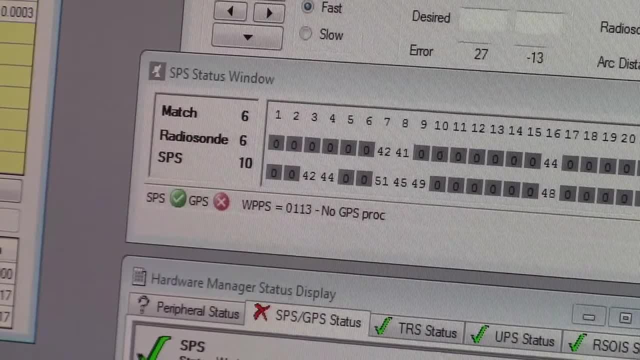 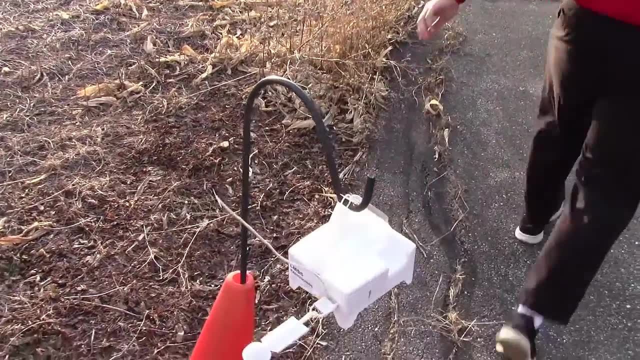 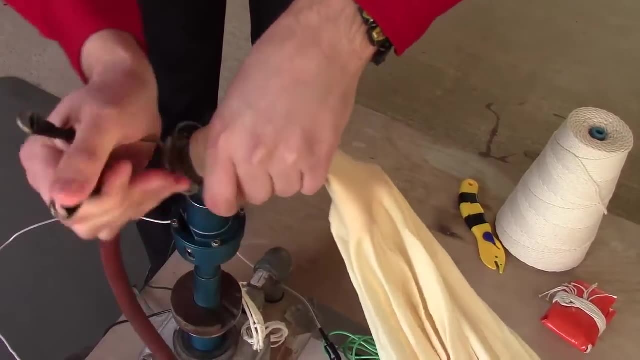 as we need a minimum of at least three for an accurate position calculation. Once we do everything in working order, we can go outside. Once the radio sign is placed at an adequate distance from the upper air shelter, we can head inside. We also want to make sure that the balloon has been inspected for deformities. 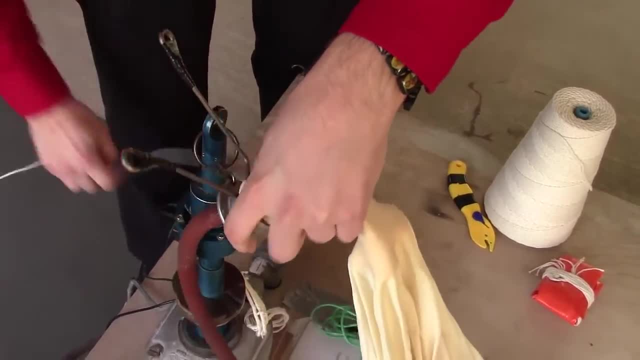 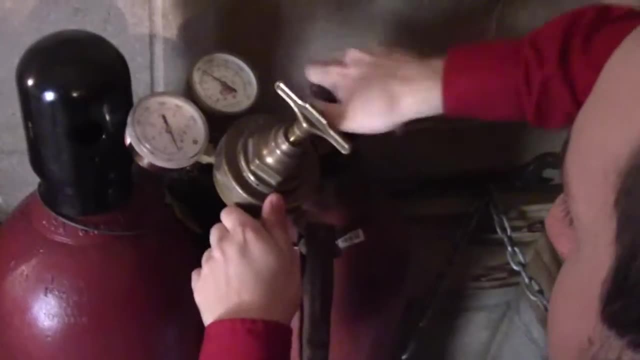 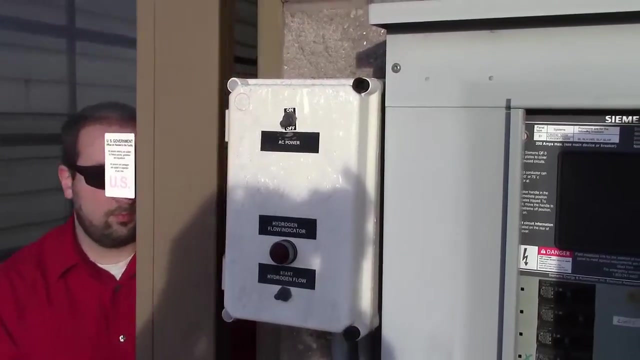 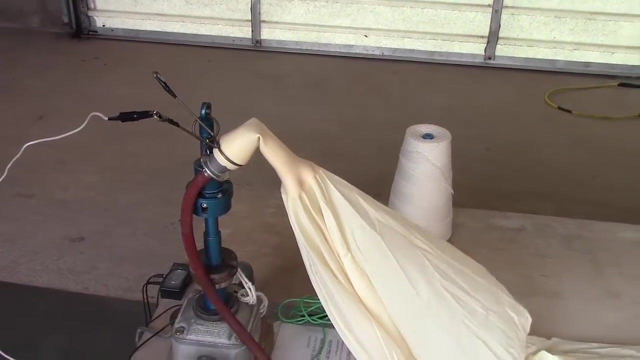 We can securely attach it to the nozzle on the inflation table. We do use hydrogen as our gas at this office, so proper precautions must be taken to ensure a safe inflation. The balloon is located at a height of 125 degrees, about 1.5 meters above the air surface. 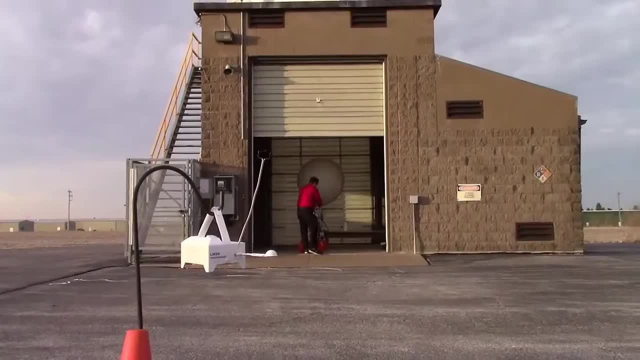 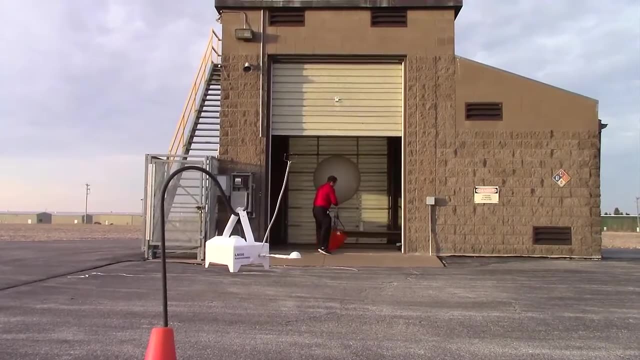 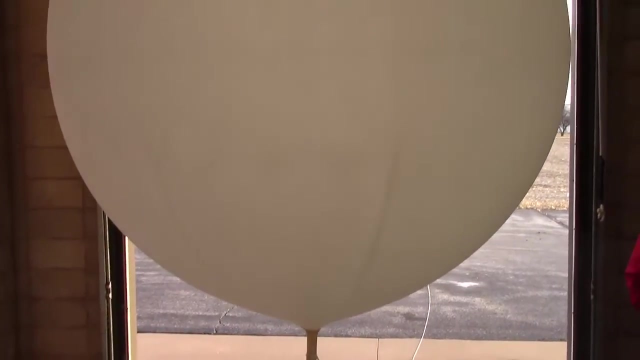 and the temperature is around 20 degrees Fahrenheit, which allows the balloon to fuel the television of the air, so there is nothing to worry about. The balloon takes roughly seven minutes to fully inflate before it rises and flips the switch to stop the flow of hydrogen. 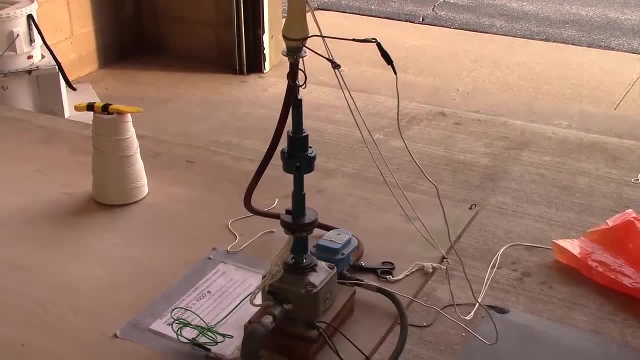 The balloon is on the air surface. In the head there is the EVA key. At this point, the balloon has been inflated. At this point, the EVA key is on the air surface. The balloon has been inflated. seal the balloon and it's officially connected to the parachute and the radio. 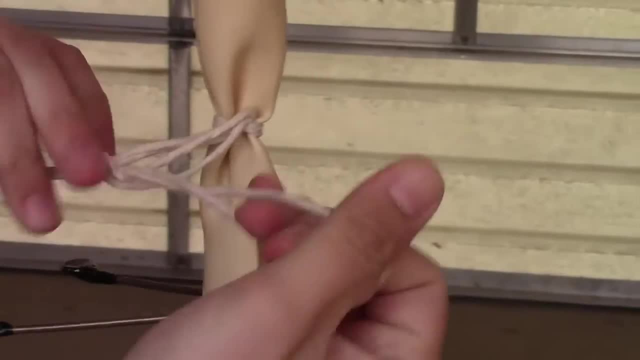 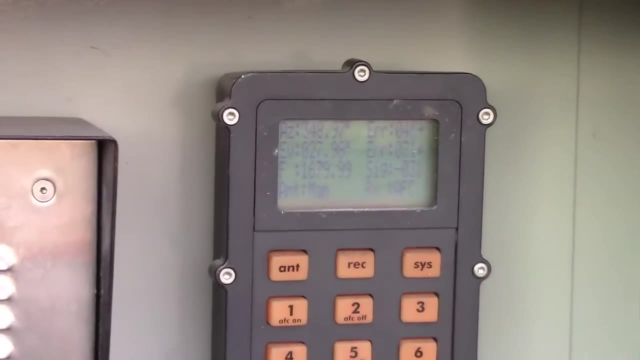 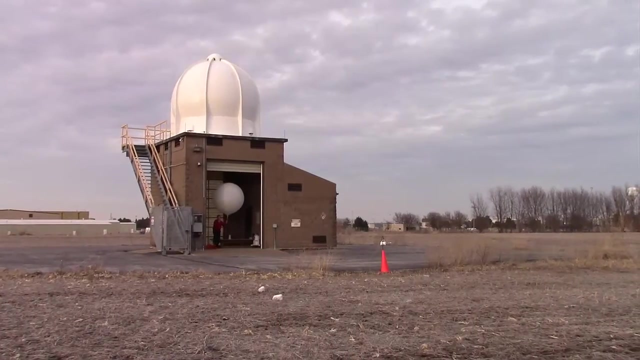 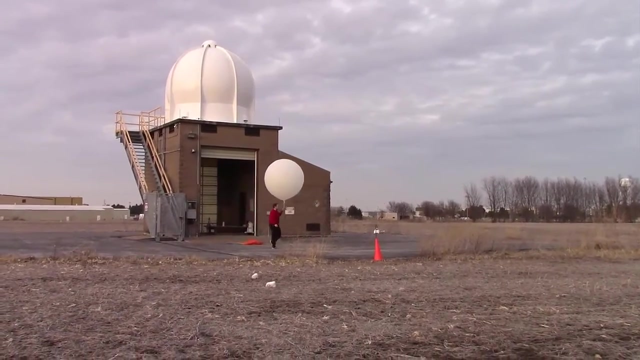 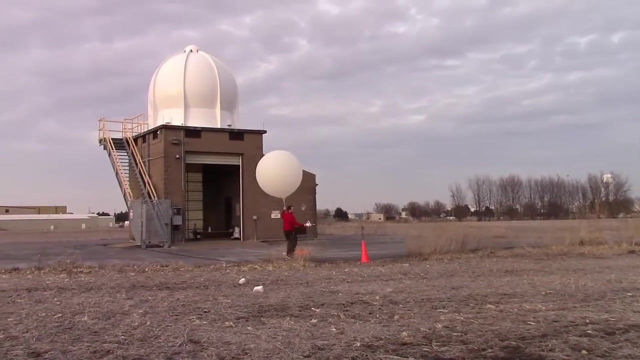 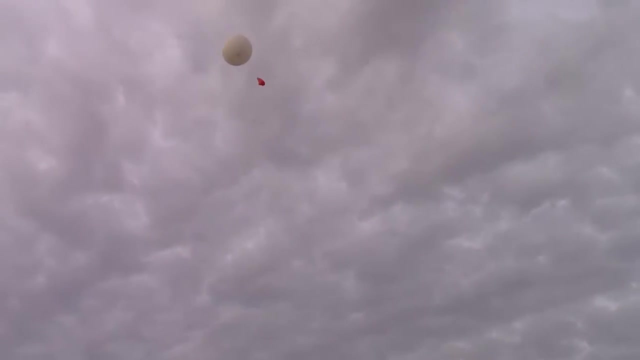 sonde. As for a neat fact, right now the balloon is roughly about six feet in diameter. After receiving clearance from the lead meteorologist inside and ensuring that all of our sensors and GPS sensors are working properly, we are ready for launch. The balloon will rise about 11 miles per hour during flight and will gradually 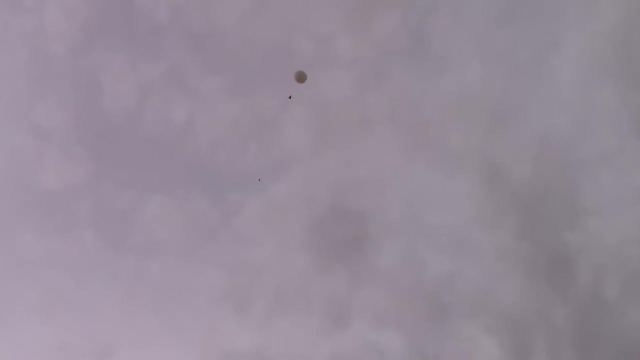 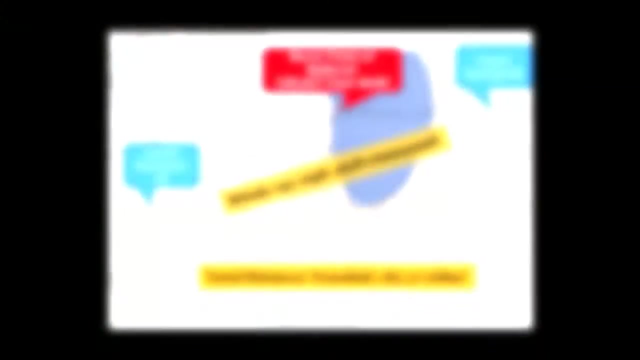 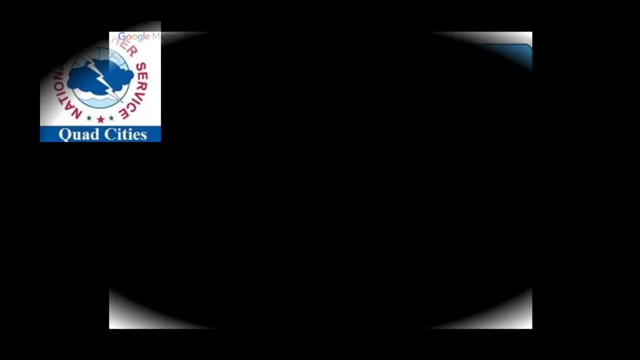 expand as the atmospheric pressure decreases. These balloons are capable of reaching heights of about 120,000 feet and can travel quite far depending on the strength of the upper-level winds. Here's one, for example. As the balloon is in flight, we perform a full quality control of the data that 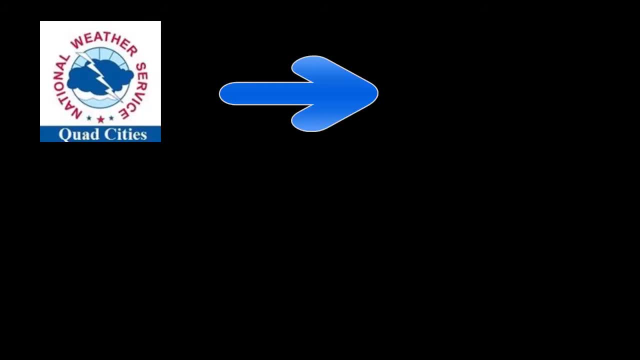 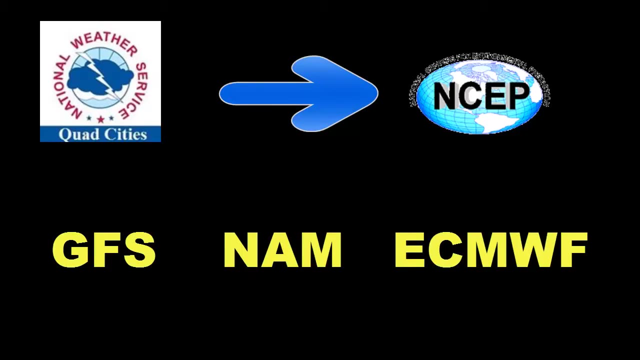 comes in. If everything looks good, then we can send off the information to the National Center for Environmental Predictions in Washington DC, which then uses this information for the evening model runs. Here's an example of what the data looks like. This is all located on the Storm Prediction Center Observed.